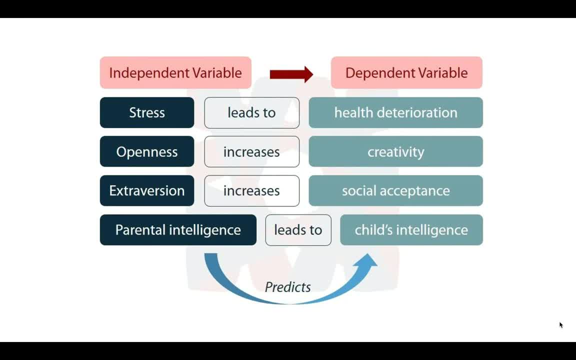 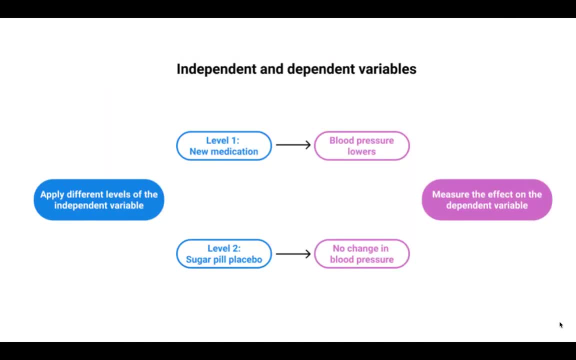 another. This is where we're going to manipulate or change one variable, which is your independent variable, And measure how it affects the other, just the dependent variable. So typically an experiment is going to have two groups: a control group that is used for a comparison who might be getting a placebo, which is like a sugar pill, and a treatment group that would be receiving the drug. 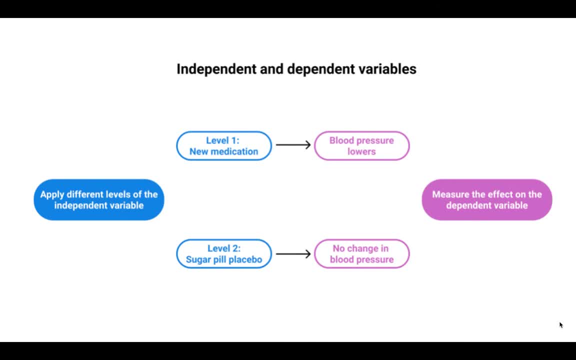 The independent variable is the one that's being manipulated. So here the independent variable is the different levels of the drug. The dependent variable is the outcome variable, in this case blood pressure, the one you're measuring to see if it's going to change. But this one is the one that's being drugged and it is going to change as a result of manipulating the independent variable. Right, And it also doesn't have to be limited to pharmaceuticals. There was an example done with some undergraduate college students where there were two groups and they were told to do sit-ups, But the one group was just told: do your best. The other group was told: try to increase your sit-ups by 10% each day, right? And both groups were measured like 100 percent each day, right? So this is where we're going to talk about how you can measure the level of sleep actually. So here's an example: the. 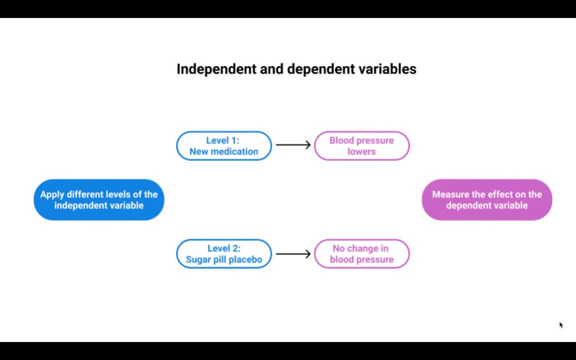 over a period of so many days And in that case the independent variable would be like the type of instruction and the dependent variable was the number of sit-ups. And, if you're curious, it did end up that the group that got the more specific directions of try to increase by 10%. 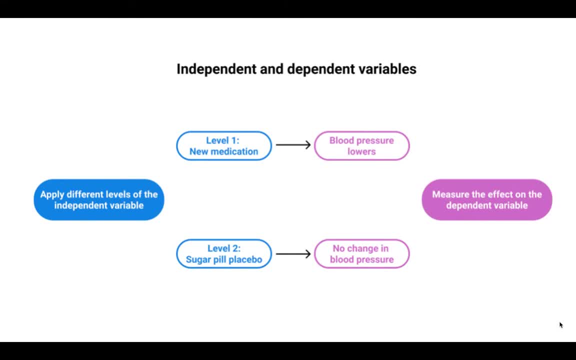 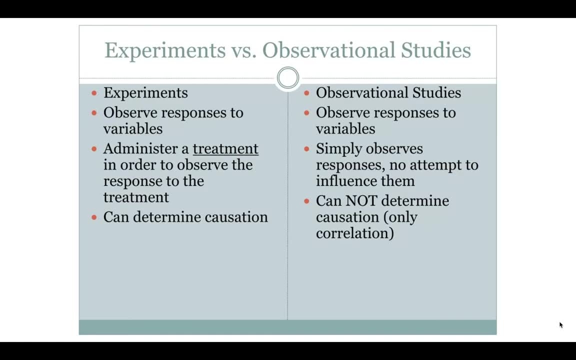 each day ended up doing more push-ups, even though both groups were randomly selected and they weren't necessarily more athletic. All right, So now we get into the observational studies. All right, This is going to draw conclusions based on observations, right, It could be data. 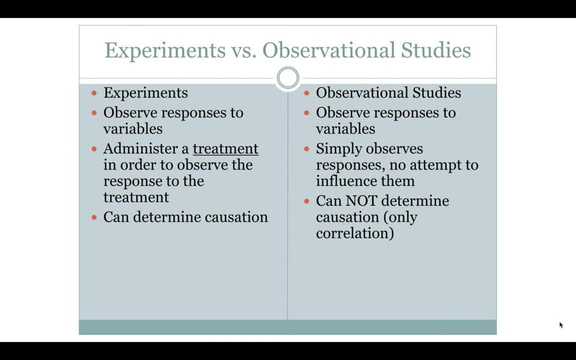 collected all at one time. It could be collected over a period of time. It could be past data that already exists. So this is going to create some disadvantages too, that, like if the data was done in the past, there's no way to really ensure the accuracy of it, So there's not a lot of control. 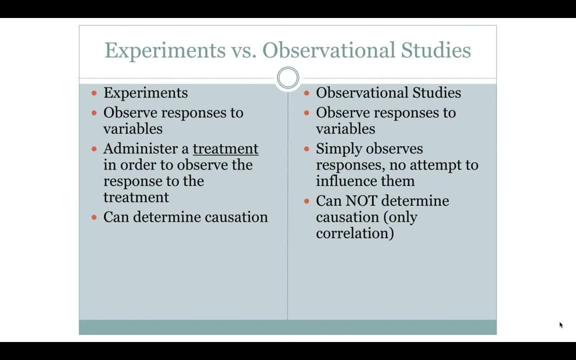 with an observational study right Besides the possibility that you could have inaccurate data and not know, and then not know it because it was previously collected, observational studies typically occur in natural settings, like not in a lab, where the researcher has more control. Observational studies could also be time-consuming and expensive, and they also don't really give a. 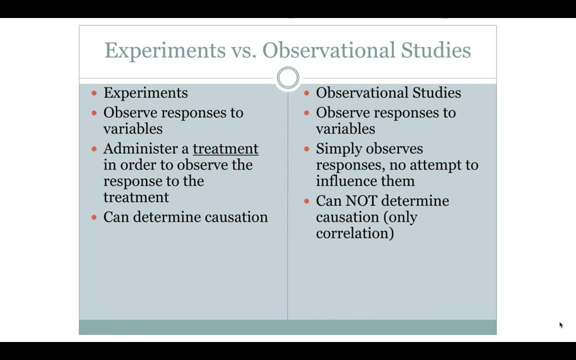 cause and effect right, Like they show correlation. They could show two things are related, but they cannot prove causation. They cannot prove that one thing causes the other. So if observational works, they call the discovery method. right, That's something that we could work on. 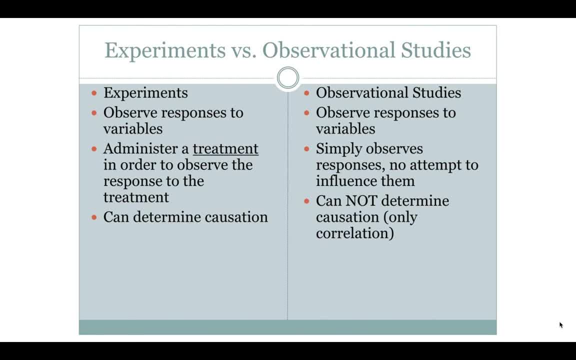 What are the advantages? Why do we even do them Right? Or when do we do them Right? we might do them if a variable cannot be manipulated or when we don't want to manipulate a variable. So an observational study would be done, maybe when it's like unethical to do an experiment, Like if you're. 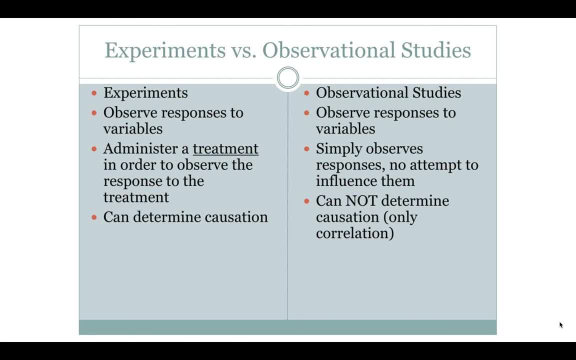 collecting data on suicide or rape or murder. obviously we're not going to experiment with collecting that type of data, But it doesn't have to be an unethical example like those It could. variable cannot be manipulated, like, let's say, I was testing whether gender 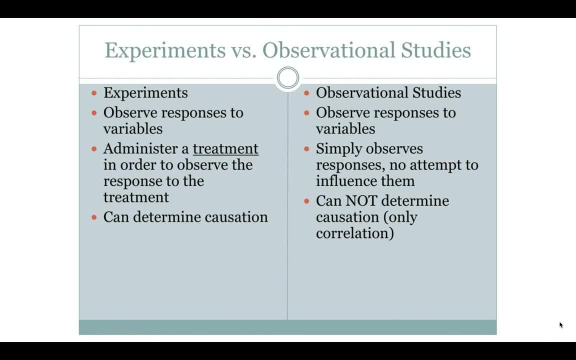 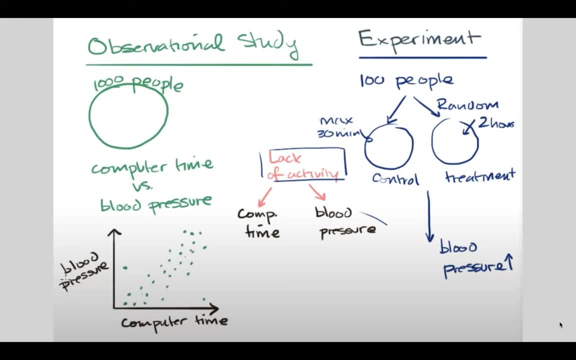 played a role in handedness, meaning like, if you're a male, are you more likely to be left-handed. suppose we have a sample of a thousand people and we're curious how people's computer time relates to their blood pressure. all right, we might ask them how much time they spend on a computer. we might record their blood. 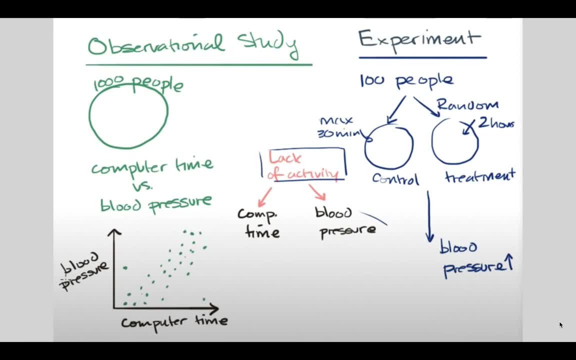 pressure. there's not going to be independent or dependent variables here because we're not measuring causation. all right, if we were just graphing the results to both of those questions and seeing how the variables like move together, right, we might be able to say that you know, higher blood pressure. 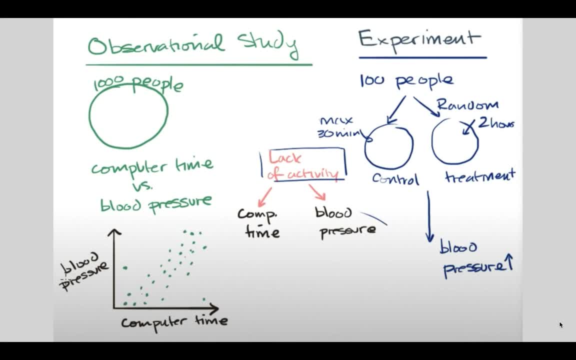 correlates with more computer time, but we would not be able to say that computer time relates to their blood pressure. all right, so we might record their blood pressure. all right, so we might be able to say that computer time causes high blood pressure in an observational study. this is because 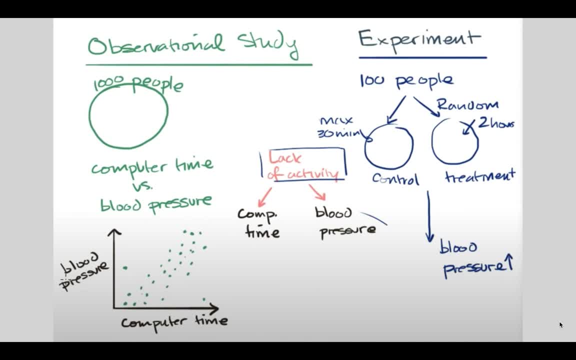 there could be something called a confounding variable that we didn't really account for, so in this case the confounding variable would be the amount of physical activity. someone has right, like typically people who are less active would have higher blood pressure, right, but people who are less active? 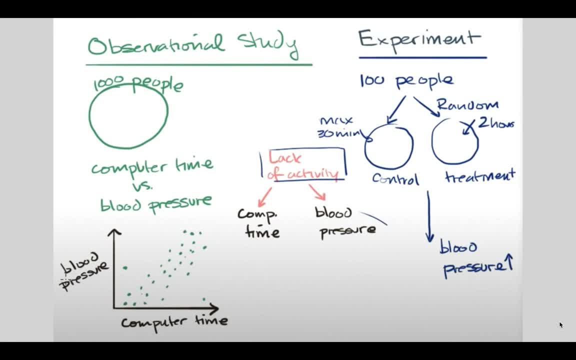 also probably have more screen time, right? so we didn't really test for that at all. so we might be able to say that computer time relates to their blood pressure, right? so we might be able to say that computer time relates to their blood outside variable. on the experiment side, if we were doing this, we would probably